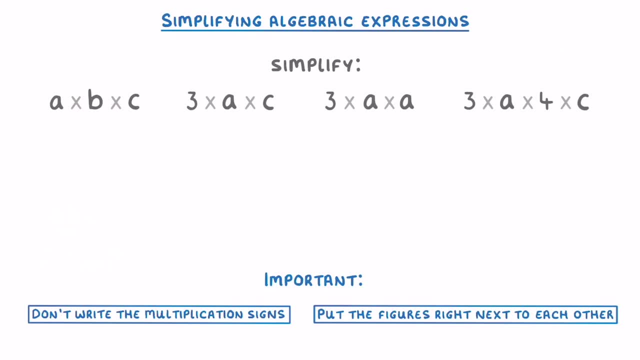 we just put the figures that are being multiplied together right next to each other. So for this first question, instead of writing a times b times c, we'd get rid of the multiplication signs so that we just have the a, the b and the c, and then we'd also get rid of the spaces in. 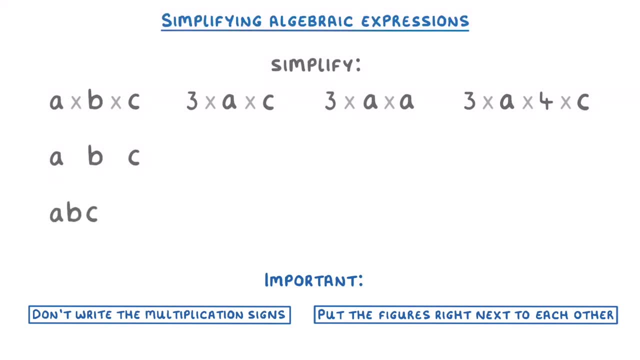 between, so that we just have a, b, c, and in algebra that means that the a, b and c are all being multiplied together. Similarly, in this next example of three times a times c, we'd just write three a c and then put them close together as three a c. It doesn't matter that we now have a number in there. we 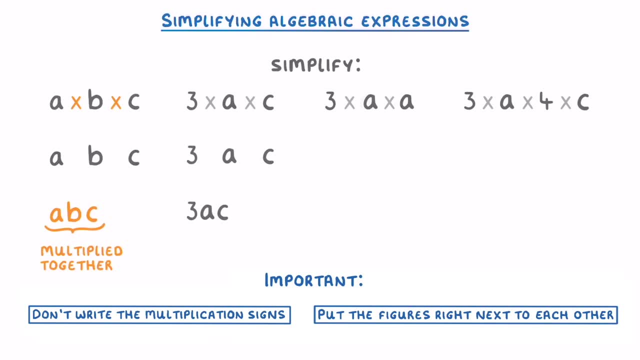 still do exactly the same thing. If you have more than one of a particular letter being multiplied together, though, like in three times a times a, then you could rewrite it as three a- a, but really we should write the a, a part, as a squared, because a squared is just a simplified version of 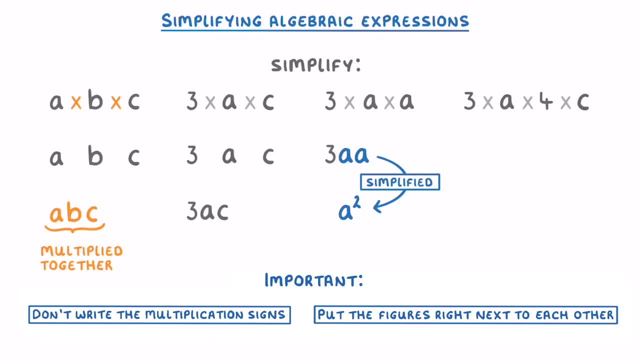 a times a, so the whole thing just becomes three a squared. In this next example we have three times a times four times c, so we have two numbers and two different letters all being multiplied together. Because they're all being multiplied, it doesn't matter which order we do it in. So this question 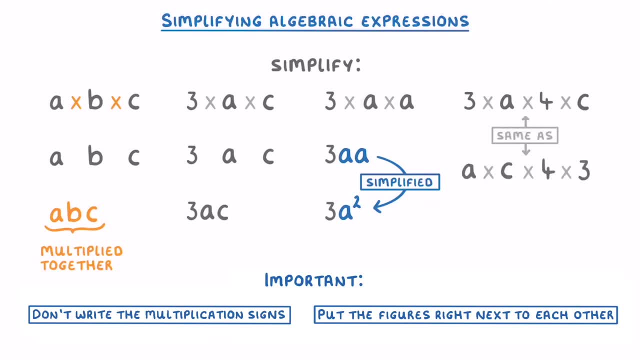 is exactly the same thing as a times c times four times three or three times four times c times a. As long as we're multiplying these four figures together, it means the same thing and we're going to get the same answer. To simplify it, though, we want to multiply the two numbers together first, so three times. 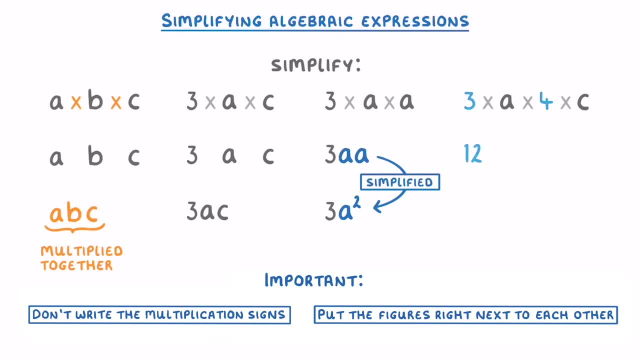 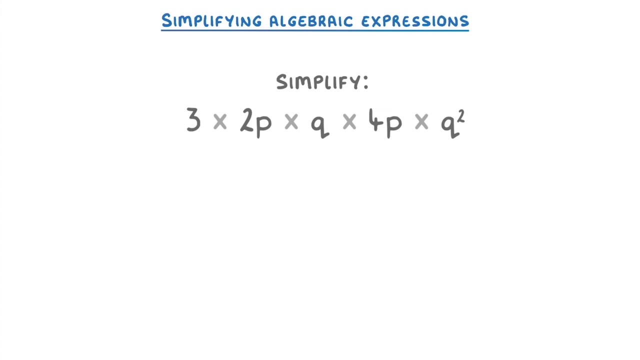 four, which is twelve, and then we can tag on the a and the c, so we end up with 12ac. Let's have a go at a slightly trickier one this time. So in this question we've got a whole bunch of numbers- p's and q's- which makes it all look a bit. 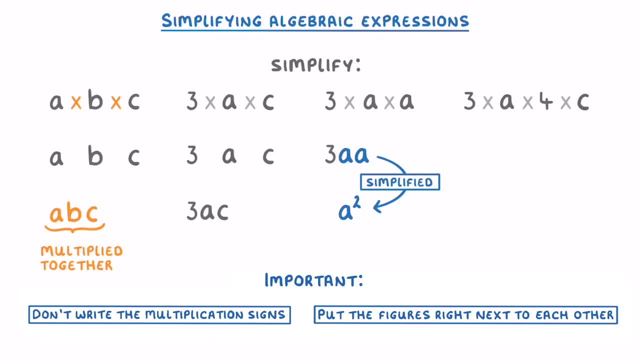 a times a, so the whole thing just becomes three a squared. In this next example we have three times a times four times c, so we have two numbers and two different letters all being multiplied together. Because they're all being multiplied, it doesn't matter which order we do it in. So this question 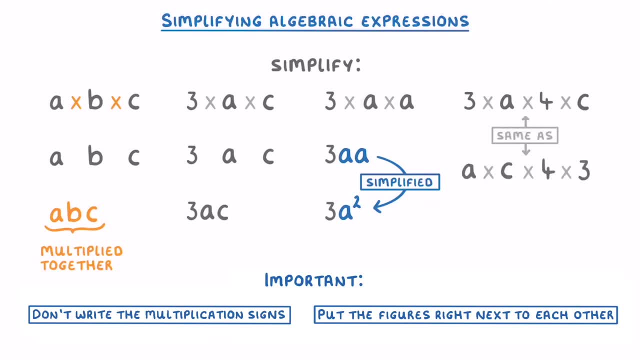 is exactly the same thing as a times c times four times three or three times four times c times a. As long as we're multiplying these four figures together, it means the same thing and we're going to get the same answer. To simplify it, though, we want to multiply the two numbers together first, so three times. 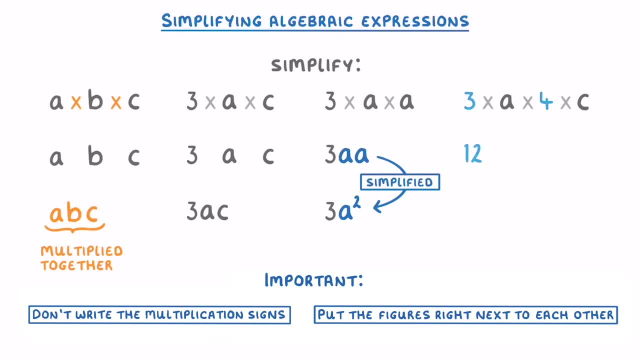 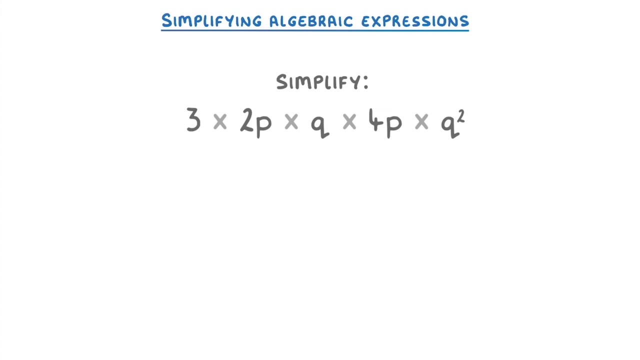 four, which is twelve, and then we can tag on the a and the c, so we end up with 12ac. Let's have a go at a slightly trickier one this time. So in this question we've got a whole bunch of numbers- p's and q's- which makes it all look a bit. 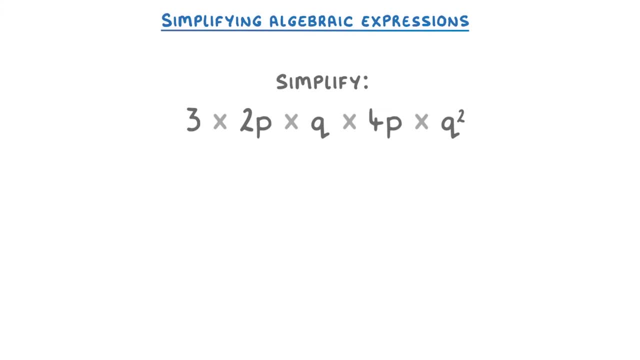 difficult. The best thing to do with these questions, though, is to think about each of these separately. So, if we start with the numbers, we have three times two times four, which is 24.. Then, moving on to the p's, we just have p times p, which is p squared. and finally, for the q's, we have 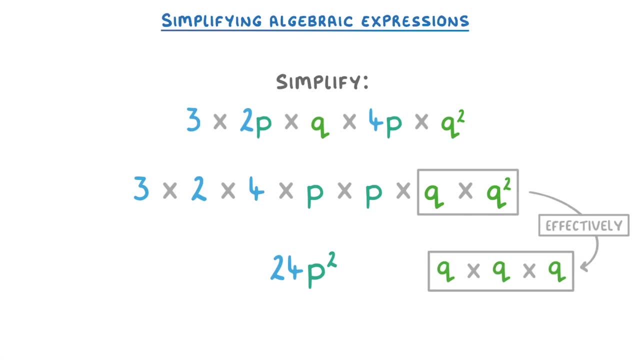 q times q squared, which is effectively q times q times q or q cubed. So overall we've simplified that entire thing down to 24p squared q cubed. For this next one, we've got minus three times minus six times a. So looking at the numbers, first we have minus three times minus six, which is 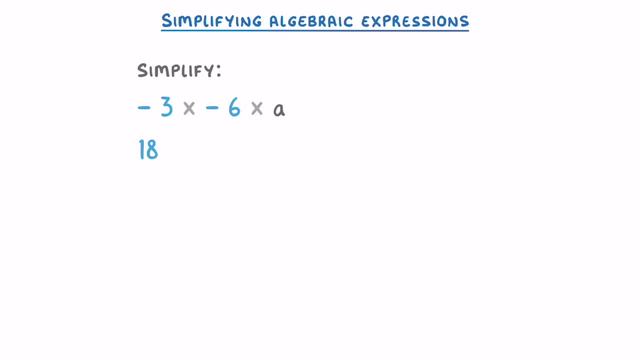 positive 18, because remember, when you multiply two negative numbers together it makes a positive number. Then we multiply the 18 by the a, so we get 18a. Now this next one negative four squared is actually a bit dodgy, because we can't. 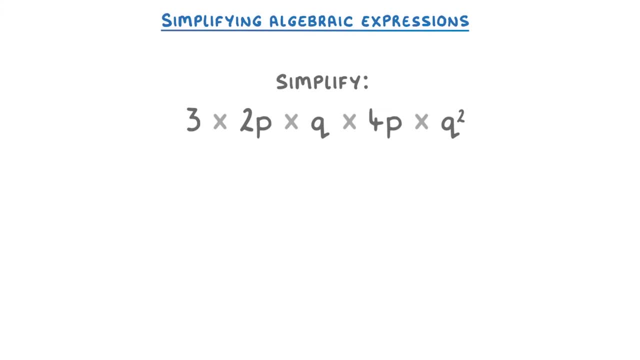 difficult. The best thing to do with these questions, though, is to think about each of these separately. So, if we start with the numbers, we have three times two times four, which is 24.. Then, moving on to the p's, we just have p times p, which is p squared. and finally, for the q's, we have 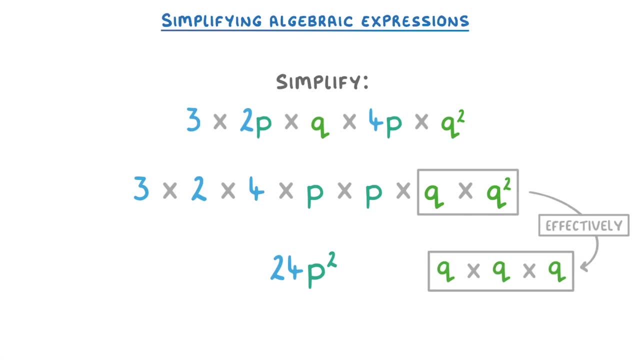 q times q squared, which is effectively q times q times q or q cubed. So overall we've simplified that entire thing down to 24p squared q cubed. For this next one, we've got minus three times minus six times a. So looking at the numbers, first we have minus three times minus six, which is 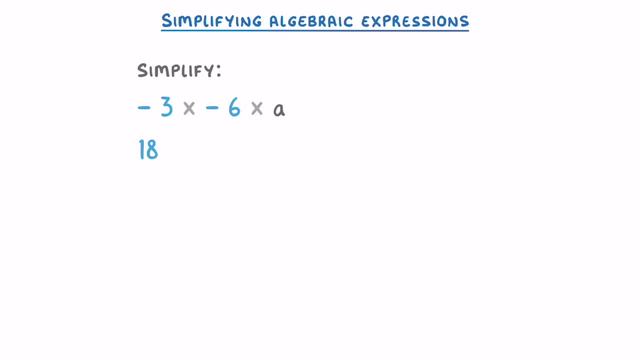 positive 18, because remember, when you multiply two negative numbers together it makes a positive number. Then we multiply the 18 by the a, so we get 18a. Now this next one negative four squared is actually a bit dodgy, because we can't. 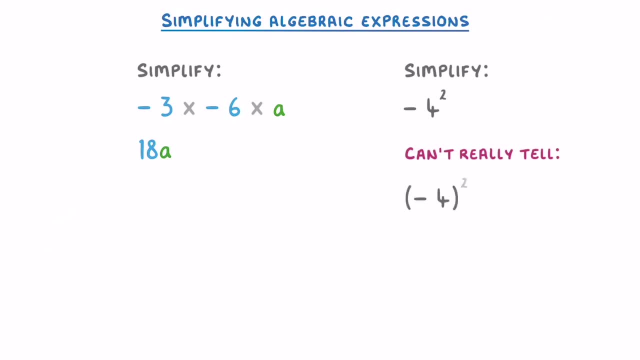 really tell whether they want us to take negative four and square it, which would be negative four times negative four, so positive 16.. Or do the negative of four squared, which would mean squaring the four to get 16, and then taking its negative, so negative 16.. In your exam they won't give you dodgy. 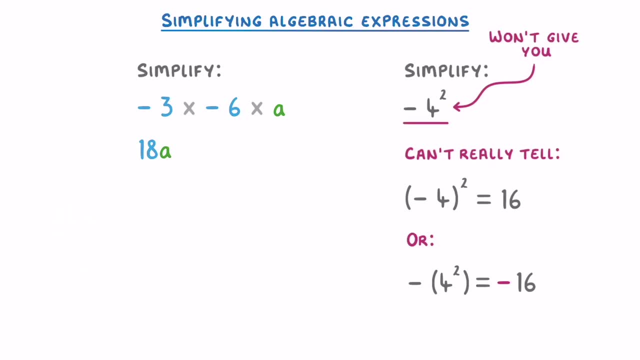 questions like this, They'll be clear about which version they want. The important point, though, is that in your own working, you need to be careful to use brackets correctly, and you need to be careful to use brackets correctly and avoid this sort of mistake. Now, sometimes you might need to expand an expression before you can simplify it. 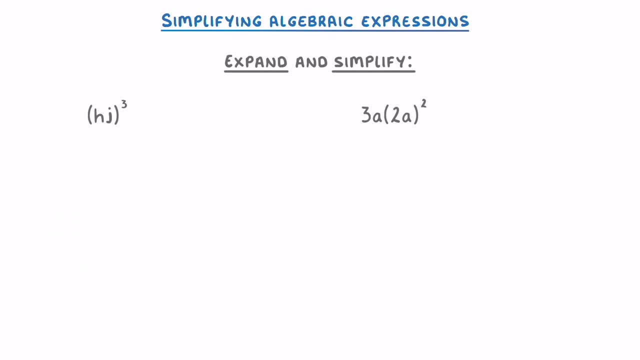 and for these questions they'll normally ask you to expand and simplify. For example, in this first one of h j cubed, we effectively have h times j inside the bracket and the cubed part means that we need to multiply the whole thing by itself to get a negative four squared. So we need to multiply the whole thing by itself to get a negative four squared. 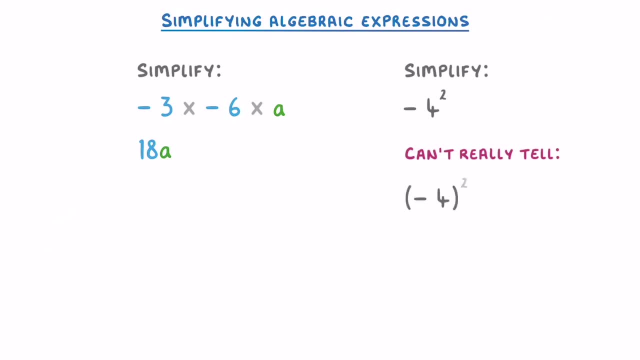 really tell whether they want us to take negative four and square it, which would be negative four times negative four, so positive 16.. Or do the negative of four squared, which would mean squaring the four to get 16, and then taking its negative, so negative 16.. In your exam they won't give you dodgy. 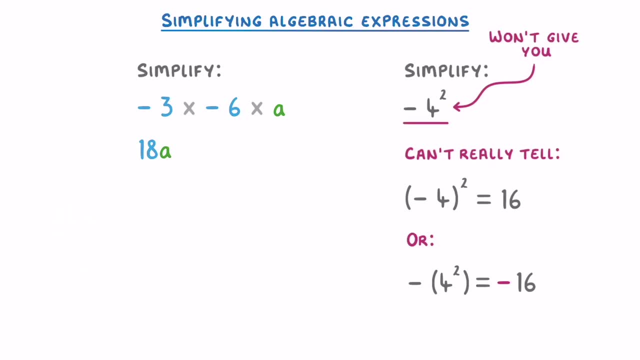 questions like this, They'll be clear about which version they want. The important point, though, is that in your own working, you need to be careful to use brackets correctly, and you need to be careful to use brackets correctly and avoid this sort of mistake. Now, sometimes you might need to expand an expression before you can simplify it. 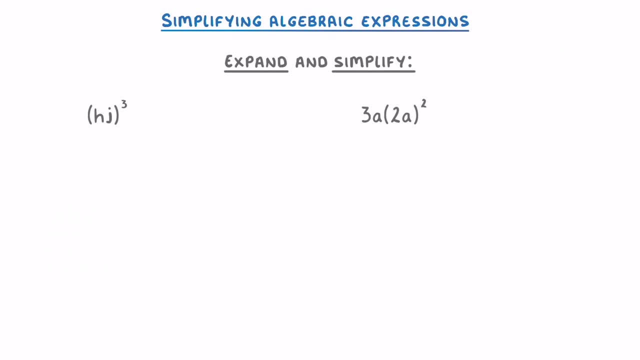 and for these questions they'll normally ask you to expand and simplify. For example, in this first one of HJ cubed, we effectively have H times J inside the bracket and the cubed part means that we need to multiply the whole thing by itself to get the same number of times j squared. 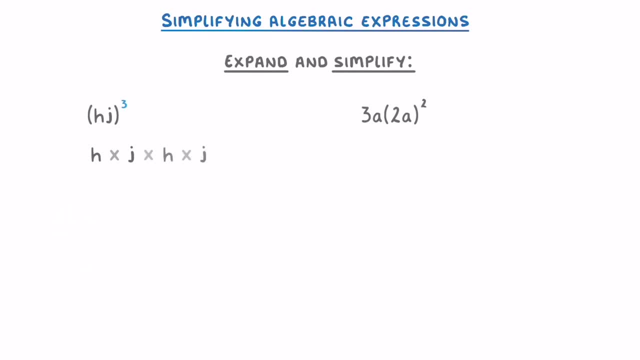 So we'll have three times. So h times, j times, h times, j times, h times j. And now that we've written it all out, we can think of the h's and the j's separately. So we have h times, h times, h, which is h, cubed times, j times, j times j, which is j. 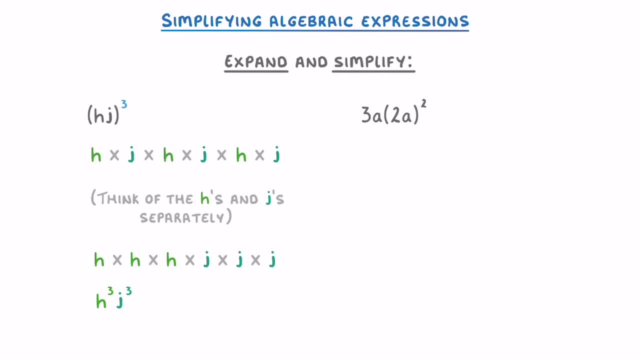 cubed. So overall it's equal to h cubed, j cubed. For this last question, we've got to. We've got 3a times 2a squared. The first thing we want to do here is expand these brackets So we can change the 2a squared to 2a times 2a, leaving us with 3a times 2a times 2a. 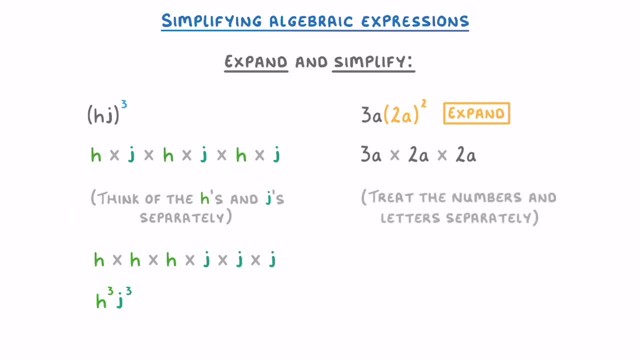 Next, we can do the same thing as usual and treat our numbers and our letters separately. So look at the numbers first. We have 3 times 2 times 2.. Which is 12.. And looking at the a's, we have a times a times a. 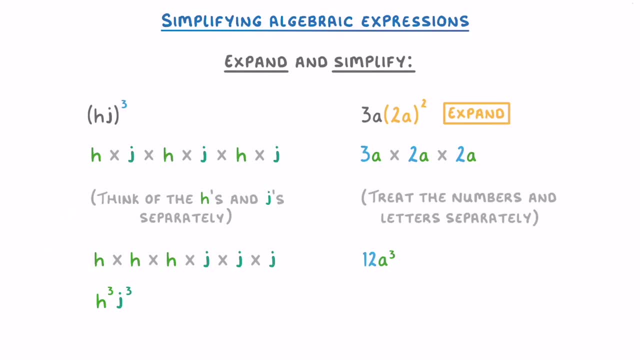 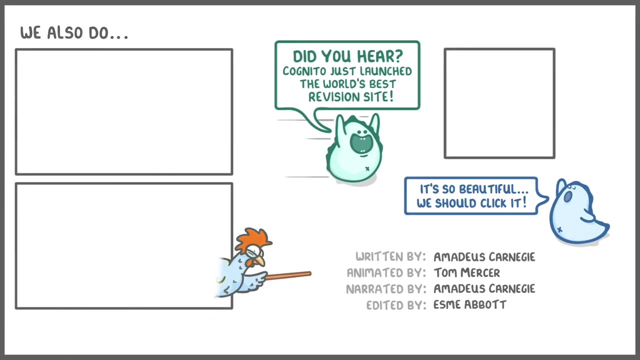 Which is a cubed. So overall we've got 12a cubed. Anyway, that's everything for this video, So I do hope you found that useful. If you did, then please do leave us a like and subscribe, And hopefully we'll see you again soon.